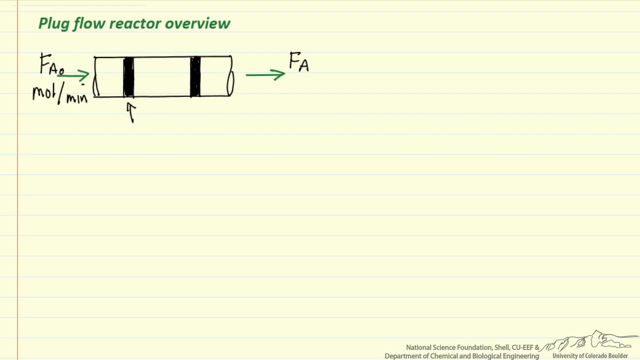 that we have a plug that's essentially moving through the reactor. It does not interact with the material in front of it. It does not interact with the material in front of it and it does not interact with the material in front of it. It does not interact with. 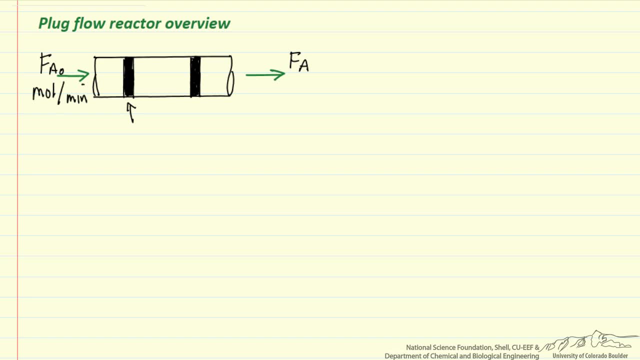 material behind it, but just moves along, and so it looks the same as a batch reactor that spends a certain amount of time, and indeed the equations for a plug flow reactor are equivalent to the equations for a batch reactor, So it's similar to a batch reactor. and what? 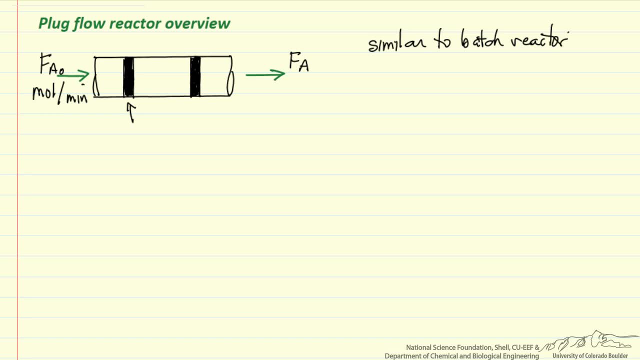 this means is that each plug has the same history, same temperature and pressure history, and it also means all molecules spend the same time in the reactor. And this is particularly important when we compare a plug flow reactor to a CSTR, where CSTR molecules don't all. 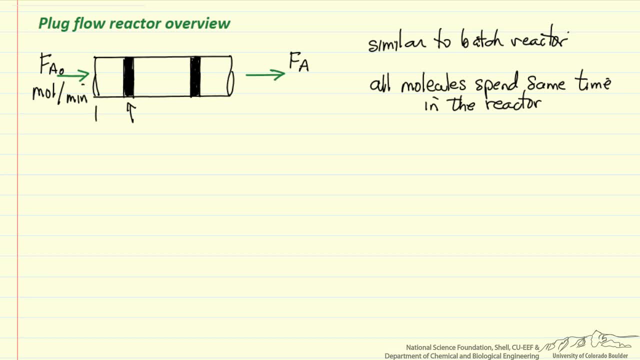 spend the same time in the reactor. So when we look at modeling this we'll use volume as our independent variable and say volume is 0 at the inlet and the outlet volume is the total volume in the reactor. So the concentration profile we're going to assume for a plug flow reactor that we 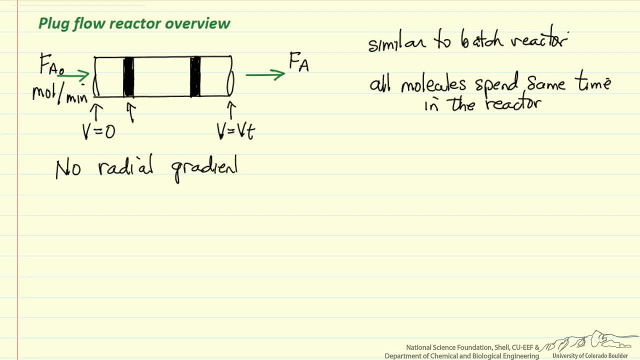 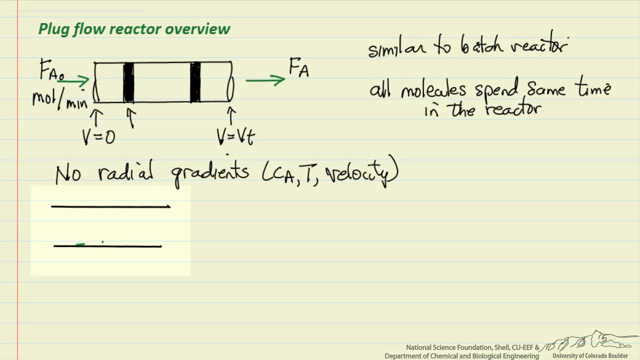 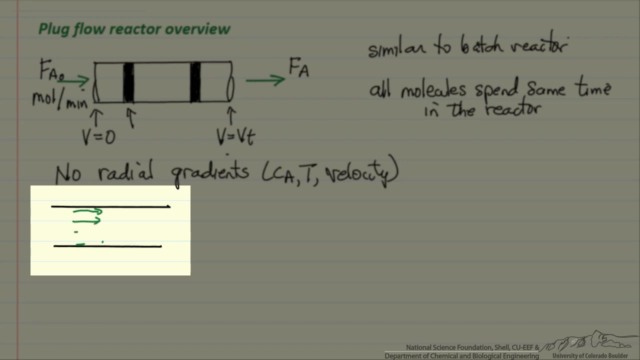 have no radial gradients. This means no radial gradients in concentration, in temperature and in velocity. So that means that if we look at a plug flow reactor, the velocity near the wall same as the velocity here, the same as here, and so we have a plug. So 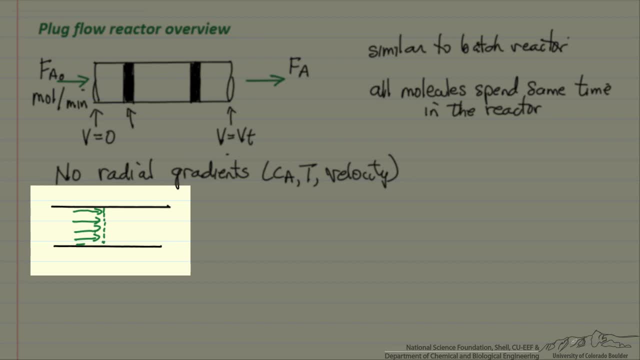 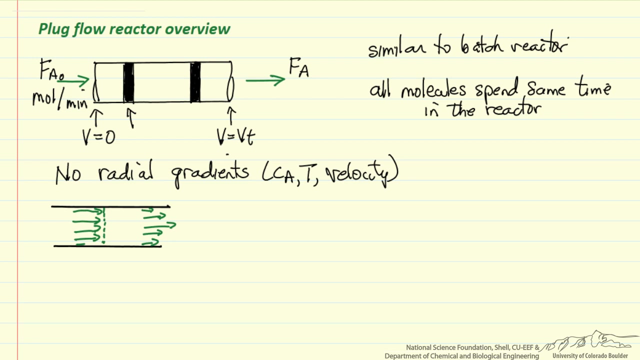 this is in contrast to a laminar flow reactor, where the velocity would be low near the wall and get bigger in the center and again lower near the wall. in a parabolic flow. It turns out a plug flow reactor is not a bad approximation to a laminar flow reactor. This 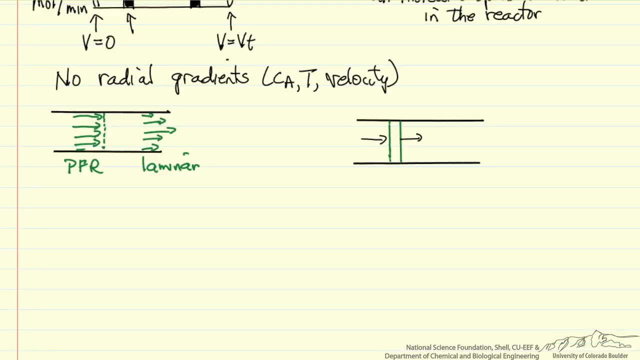 is plug flow reactor. this is laminar. In order to write down the mole balance for a plug flow reactor, we look at a differential volume. We have flow rate and we have the flow rate in and the flow rate leaving is different because of reaction and we write. 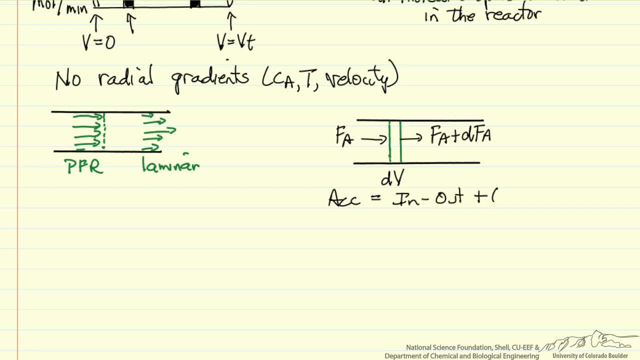 the mass balance: accumulation in minus out, plus generation due to reaction. We're interested in steady state, so accumulation is 0, we're going to do a balance of 1 component, so that's A in this case, in minus out, and the generation is some rate of reaction in this differential. 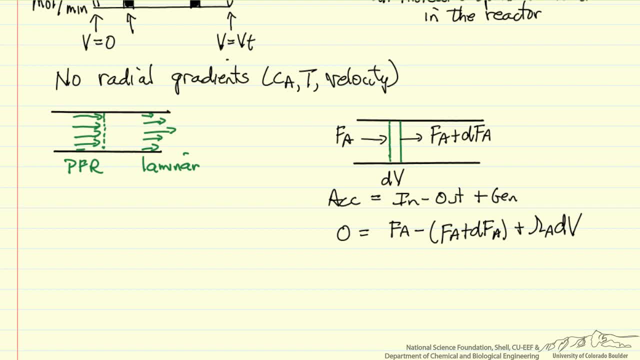 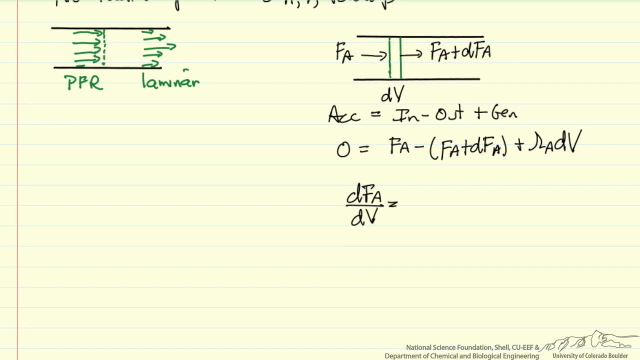 volume. So the rate of reaction is 0.. is per volume, so we multiply by the differential volume and this simplifies to the change in the molar flow rate with cumulative volume. is r sub a, where r sub a might be k concentration. 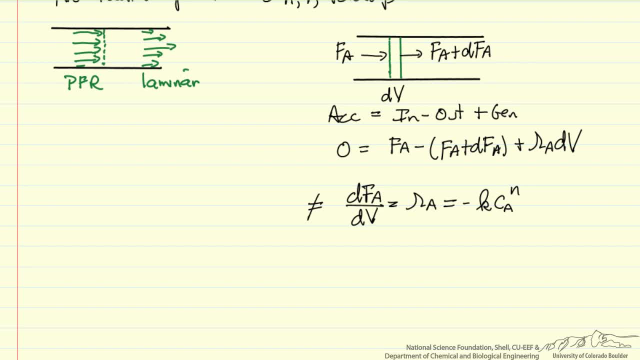 of a raised to some power. What we're not going to do is write it this way because, remember, the molar flow rate is the volumetric flow rate times the concentration. this is moles per minute, volumetric flow rate, for example, liters per minute, and concentration. 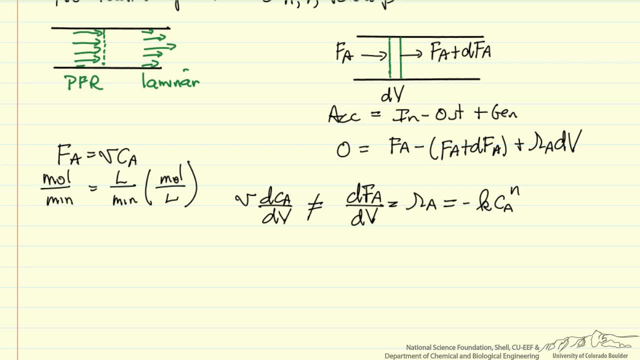 moles per liter. We're not going to do this because the volumetric flow rate changes. It changes because the temperature changes, because the pressure changes and because the moles change, namely if A in the gas phase reacts to form two moles of gas per liter. 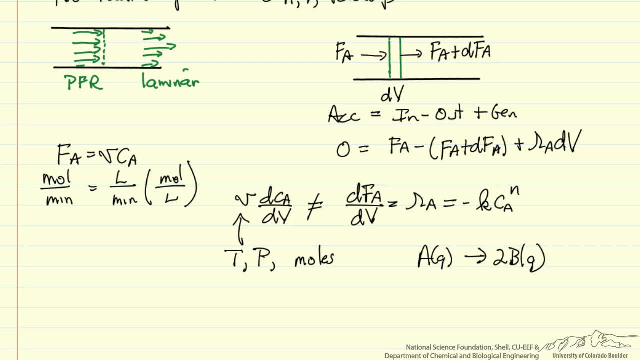 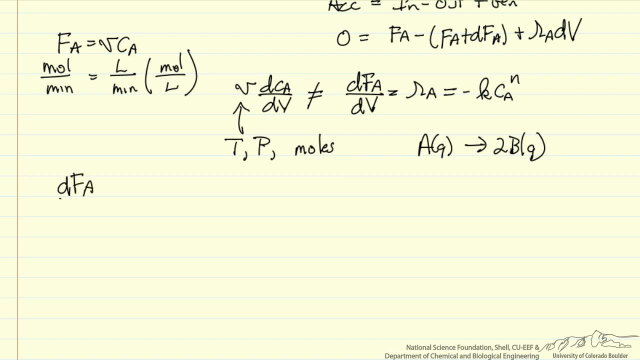 So B, in the gas phase we increase the number of moles. this changes the time in the reactor. Now there are other ways we can write this mass balance, the change in the flow rate respect to z, and I'll just bring the cross sectional area. so the equation otherwise is: 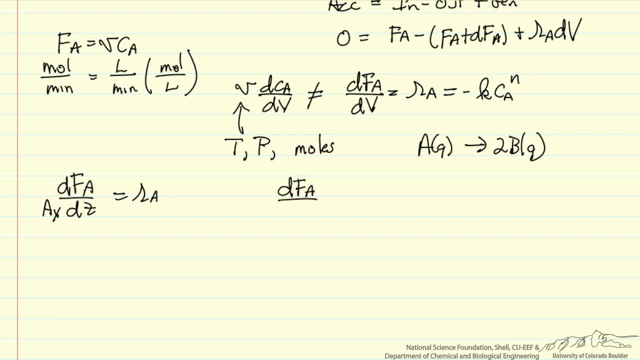 the same, or I could write it in terms of the cumulative amount of catalyst, the weight of catalyst. So I'll write this rA prime, because now we have units of moles per minute, for example, per kilogram of catalyst on both sides of. 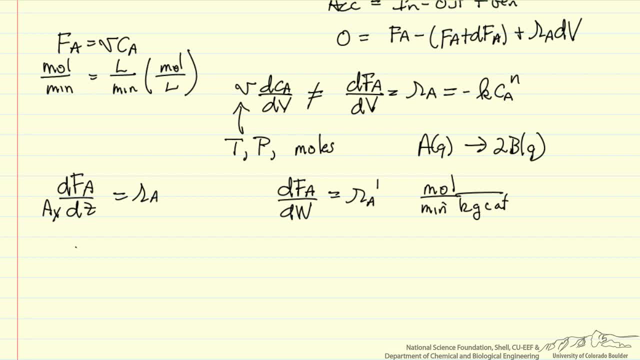 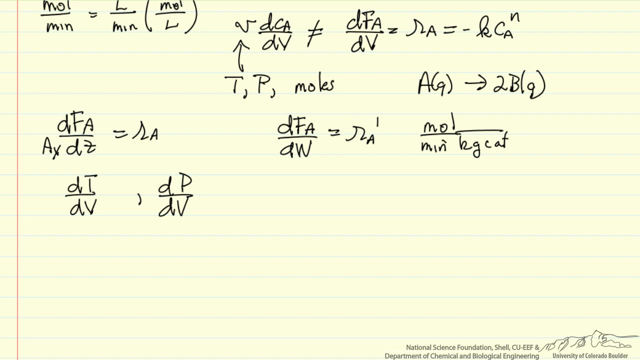 the equation. In addition to solving the mass balance, we'd also have equations for energy balance, equations for pressure, and we could write a mole balance for each of the species in the plug flow reactor. So why would we use a plug flow reactor? So here's when we